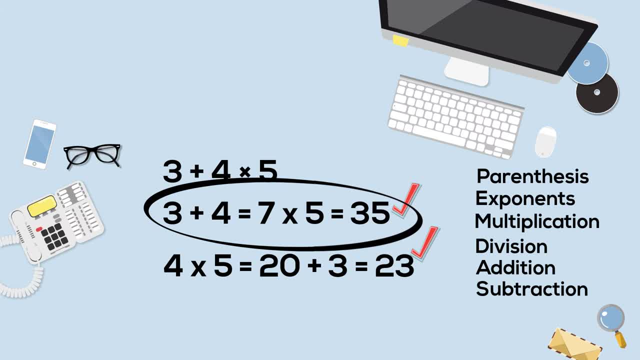 times 5 equals 35.. The second answer is 23, and that is the correct answer. The second answer is 23 and that is the correct answer. The first one you have: 3 plus 4, which equals 7 times 5, equals 35.. 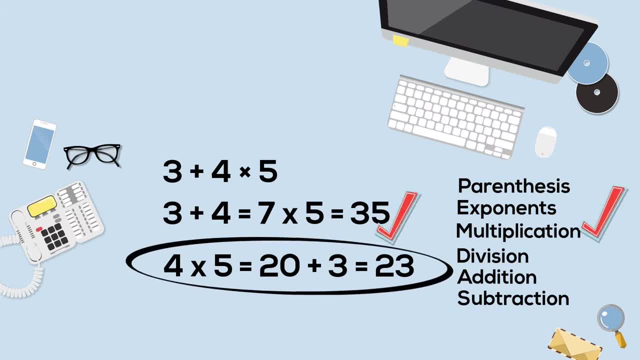 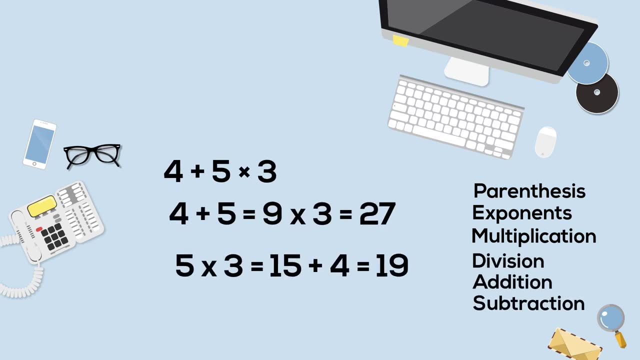 You follow the order of operation. You multiply first 4 times 5, which is equal to 20, and then you complete addition. So the correct answer is 23.. Let's look at this next example. Which answer is correct? 27 or 19? 27? you take 4 plus 5, which is 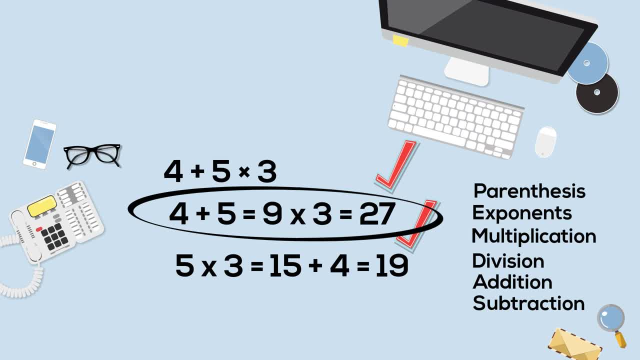 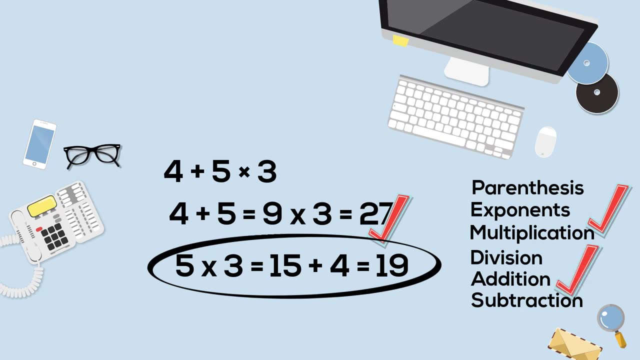 equal to 9. then multiply that by 3, which is equal to 27.. So you're just going from left to right. The correct answer is 19.. You first complete multiplication, which is 5 times 3, which is equal to 15.. Then you complete addition, and that is 19.. Remember PEMTAS. Follow that for. 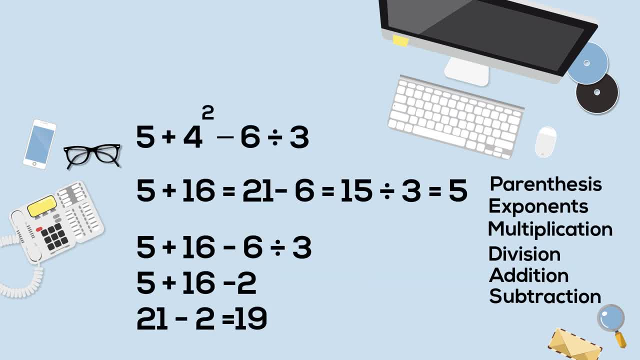 the correct order of operations. And for the last one, Which is correct, 5 or 19?? And this has exponents. The first example, I will just work from left to right: 5 plus 4 squared, which is 4 squared. 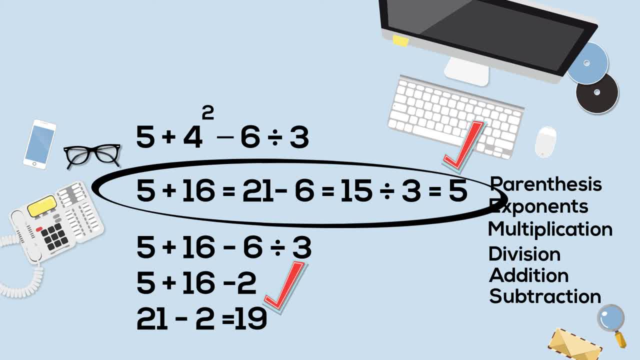 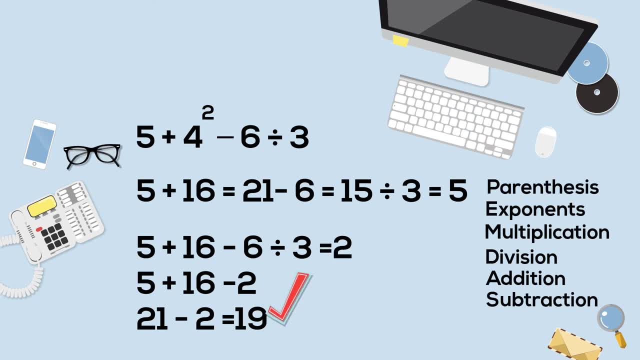 16 is 21.. Subtract 6. That equals 15.. Divide by 3 and that equals 5.. The correct answer is 19.. Let's see the difference. First let's work exponents. So 4 squared is 16.. 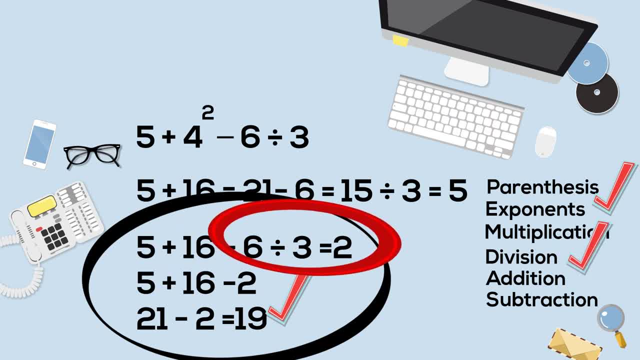 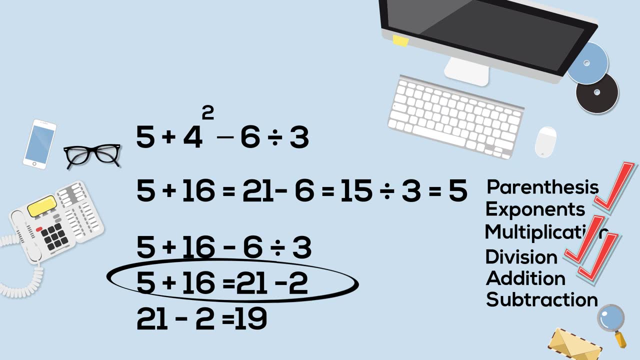 Next you complete division. So 6 divided by 3 is 2.. And now you move down PEMTAS. and next is addition: 5 plus 16 is 21.. And finally, complete subtraction: 21 minus 2 equals 19.. So there's the correct answer. 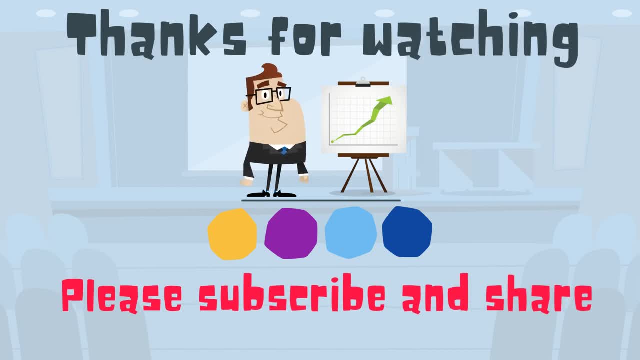 Thanks for watching, and MooMooMath uploads a new math and science video every day. Please subscribe and share.